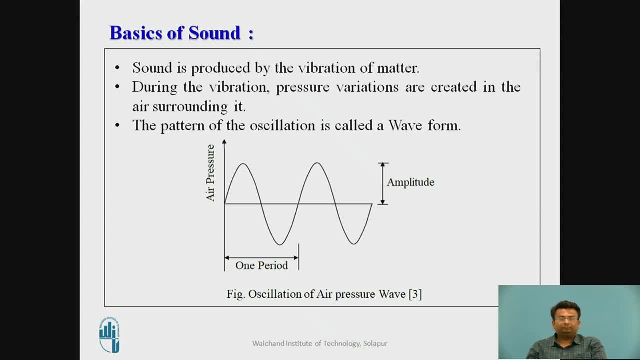 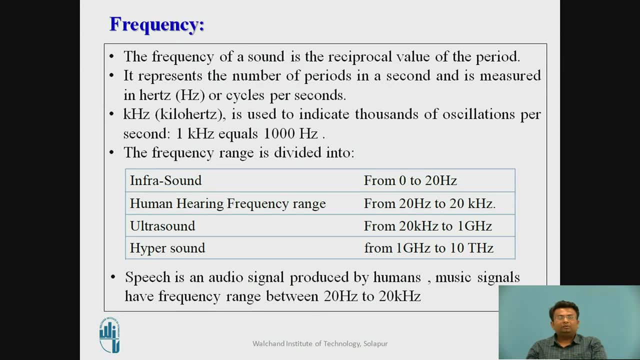 to it. The pattern of this oscillation is called as a waveform. The waveform repeat itself after the particular time of the interval which is called as a one period. Let us move to the frequency. The frequency of the sound is reciprocal value of the period. It represents the number of 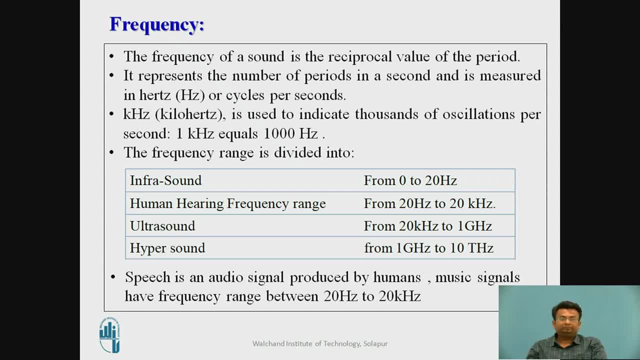 periods in second, and it is measured in hertz or cycle per second. Kilohertz is used in order to indicate thousands of oscillations per second. That means 1 kilohertz will be equal to 1000 hertz. The frequency ranges are divided into infrared sound. It varies from 0 to 20 hertz. 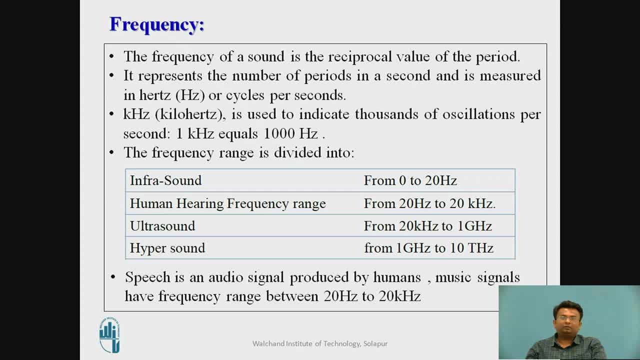 The human hearing frequency ranges from 20 hertz to 20 kilohertz, The ultrasound ranges from 20 kilohertz to 1 gigahertz and the hypersound ranges from 1 gigahertz to 10 terahertz. A speech is an audio signal which is produced by the 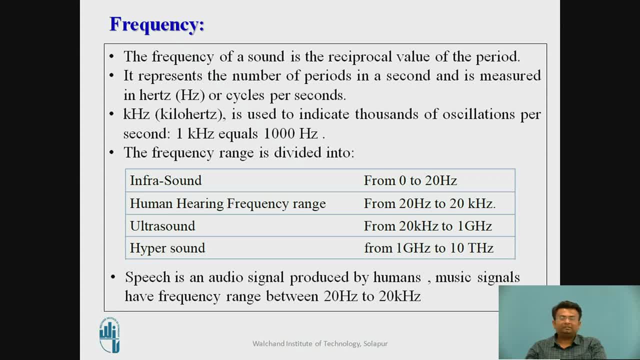 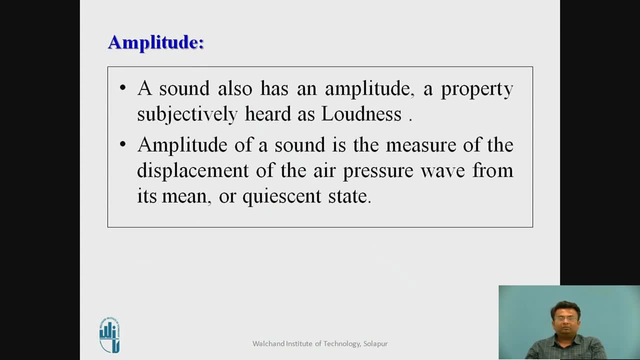 human or the music signals which have the frequency ranges in between 20 hertz to 20 kilohertz. The amplitude of the sound. The amplitude of the sound is also called as loudness. The amplitude of the sound is major of the displacement of the air pressure waveform. 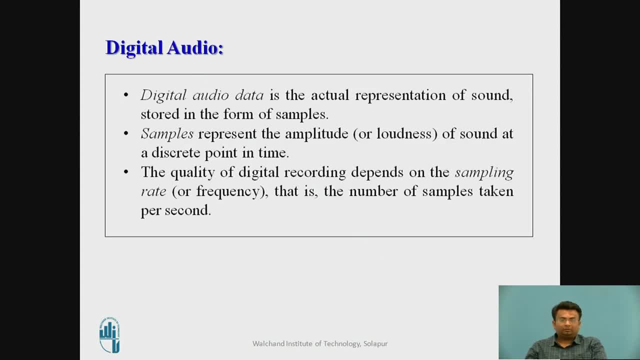 from its mean value. The digital sound. A digital audio data is actual representation of the sound which is stored in the form of samples. Samples represent the amplitude of the sound at discrete points in the time. The quality of the digital recording depends on the sampling rate, That is, the number of samples taken per second. 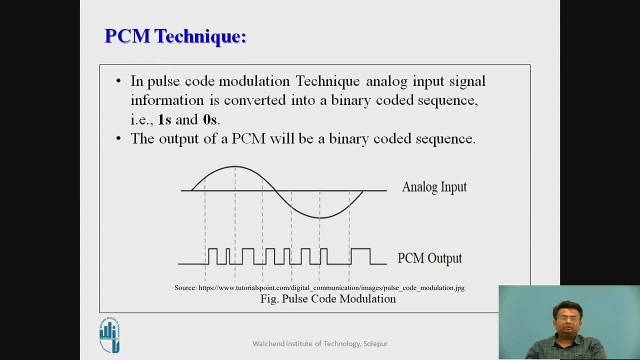 The PCM technique, which is used for the audio compression In pulse code modulation technique. the analog input signal information is converted into the binary coded sequence, That is ones and zeros. The output of the PCM will be the binary coded sequence as shown in the 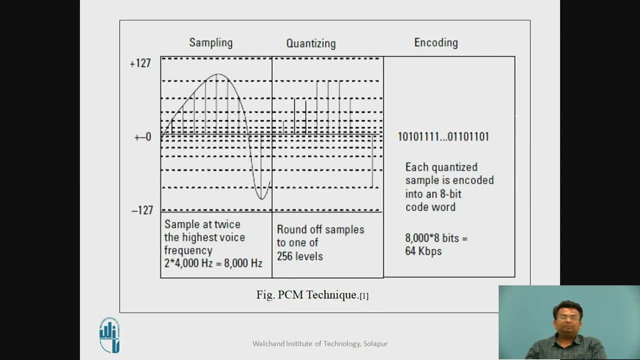 figure. The output of the PCM will be the binary coded sequence as shown in the figure. There are three main steps in the PCM technique. First is the sampling, then quantizing and then encoding. Sampling is nothing but the conversion of the analog signal into the discrete samples. 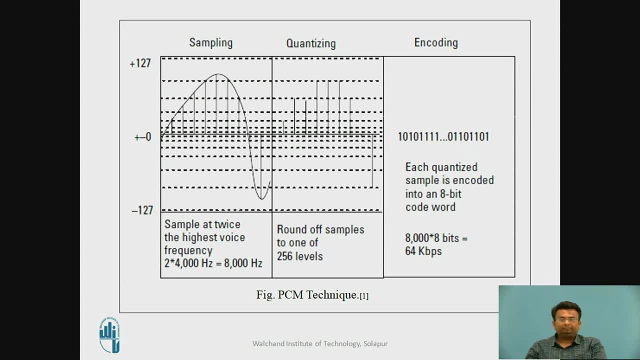 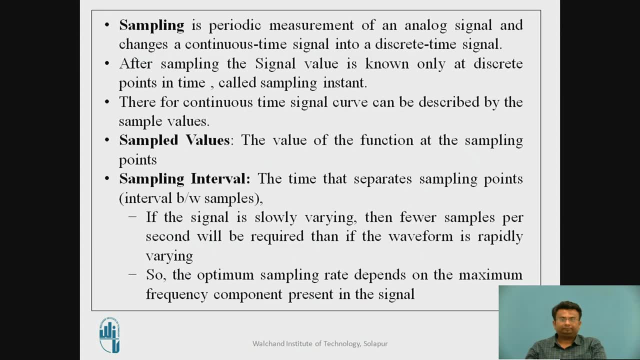 Quantization is nothing but the rounding of the samples to the nearest values, And then encoding is nothing but the each quantized samples are coded into the binary data. So let us move to the sampling. The sampling is a periodic measure of the analog signal, and it changes the continuous 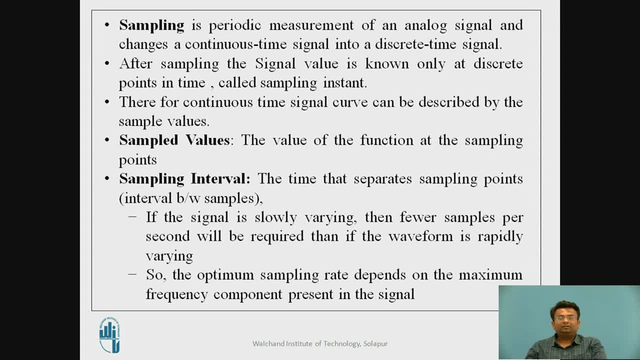 signal into the discrete time signal. After the sampling, the signal value is known only at discrete points in the time. These points are called as a sampling instant. Therefore, continuous time signal curve can be re-described by the sample values. The Sampled Values, The value of the function at sampling point. 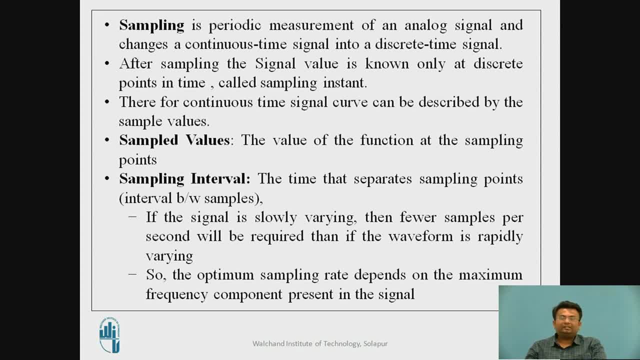 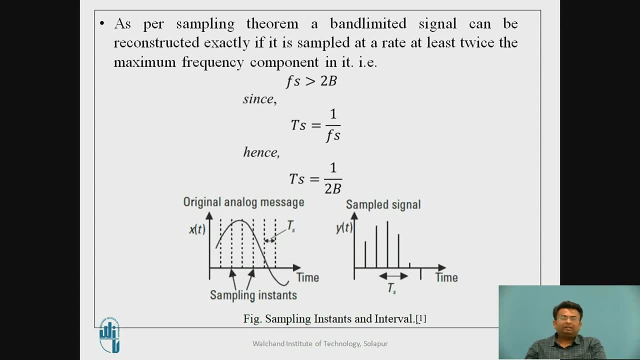 is nothing but the sampled values, The Sampling Interval, The time that separates the two sampling points, is nothing but the sampling interval. As per the sampling theorem, the band-limited signal can be reconstructed exactly if it is sampled at the rate at least twice the maximum frequency component which is present. 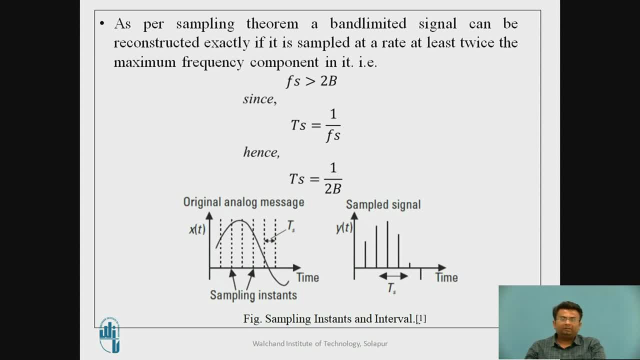 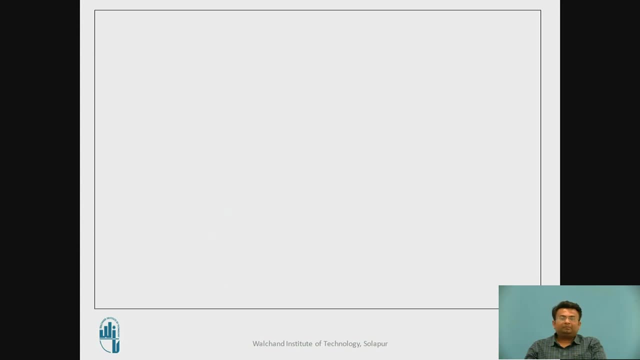 in it. That means fs should be greater than 2b. The b defines the band-limited signal bandwidth. So we know that the Ts ie time period is reciprocal of the frequency. Hence the sampling interval will be 1 upon 2b. 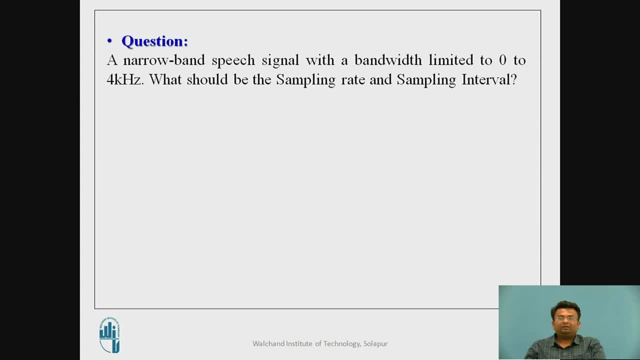 Let me ask you the question. The narrowband speed signal is limited to 0 to 4 kHz. What should be the sampling rate and the sampling interval? You may pause the video, think about this question and write your answer in a notebook. 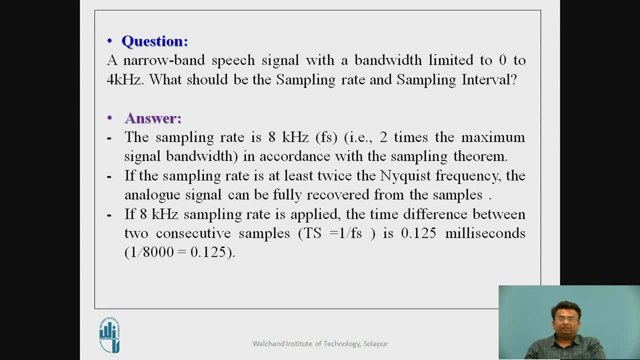 Let me answer the question. The sampling rate is 8 kHz Because, as per the sampling theorem, the sampling rate should be twice than that of the bandwidth of the baseband signal. So if the 8 kHz is the sampling rate, then the difference between the two consecutive samples 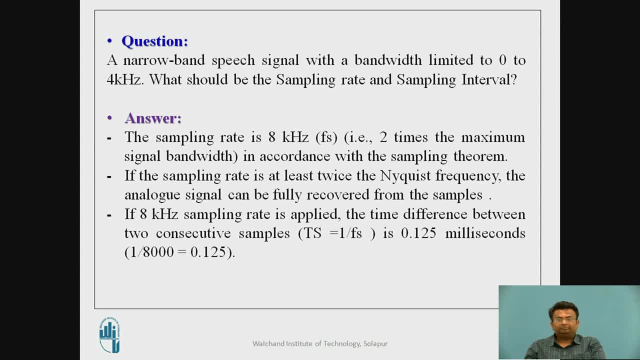 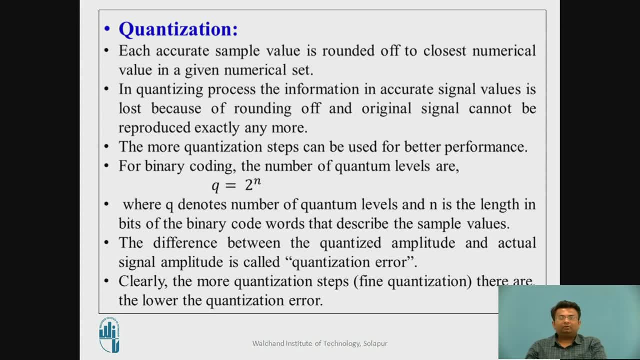 will be 0.125 ms. each accurate sample value is rounded off to the closest numerical value in the given numerical set. In quantizing process the information in the accurate signal value is lost because of the rounding of the and original signal cannot be reproduced exactly. 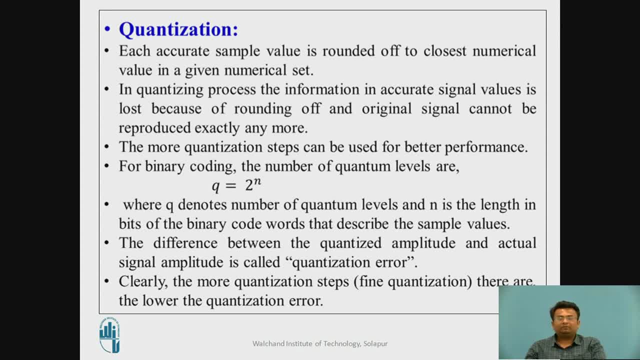 anymore. The more quantization steps can be used for the better performance For the binary coded. the number of quantum levels are defined as: q is equal to 2 raised to n, where the q denotes the number of quantum levels and n is the length in the bits of. 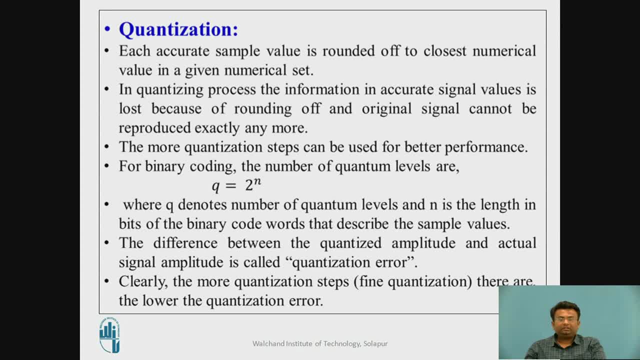 the binary words that describe the sample values. The difference between the quantizable amplitude and the actual amplitude is called as a quantization error. So more the quantization step there will be the lower quantization error. Coding The coding process will convert the discrete. 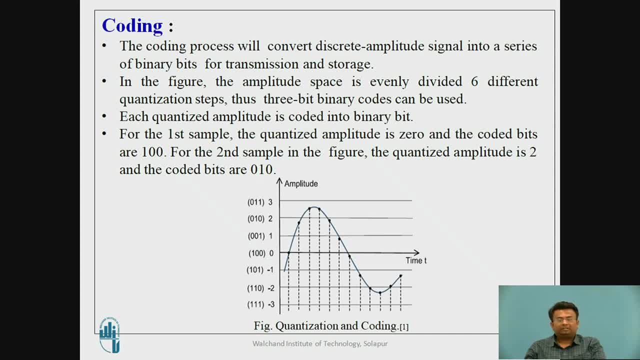 amplitude signal into the series of binary bits for the transmission and the storage. As shown in figure, the amplitude space is evenly divided into 6 different quantization steps. Thus, 3-bit binary cores can be used in order to convert this analog signal into the discrete. 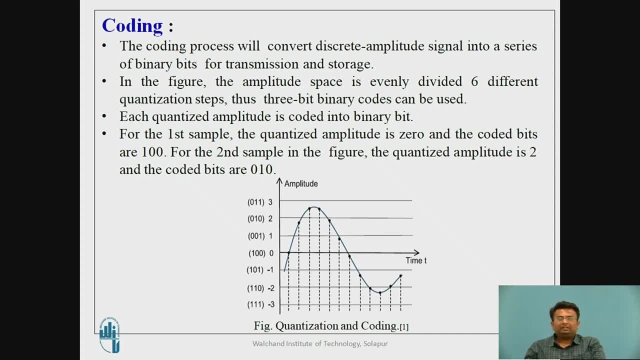 signal. So for the first sample, the quantized amplitude is 0 and it is coded bits into the 1, 0, 0.. For the second sample, The quantized amplitude is 2 and then it is coded into 0, 1, 0.. 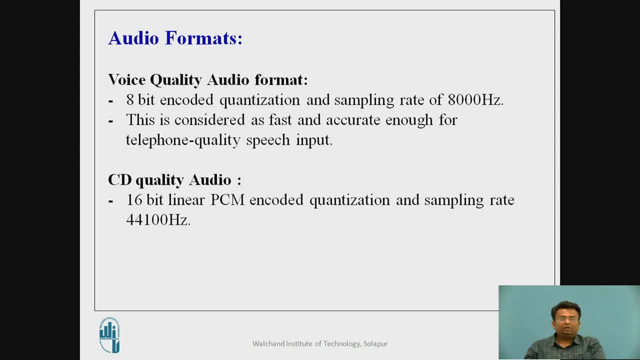 Audio formats. There are basically two audio formats: The voice quality audio format and the CD quality audio format. Voice quality audio format. In this audio format the 8-bit encoded quantization level is used and the sampling rate is 8000 Hz. This is considered as fast and accurate enough for the telephone quality speech input. 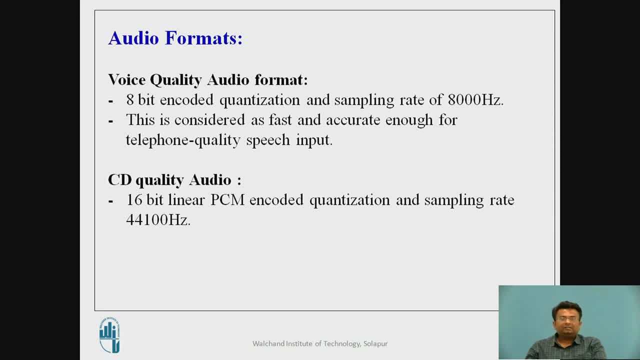 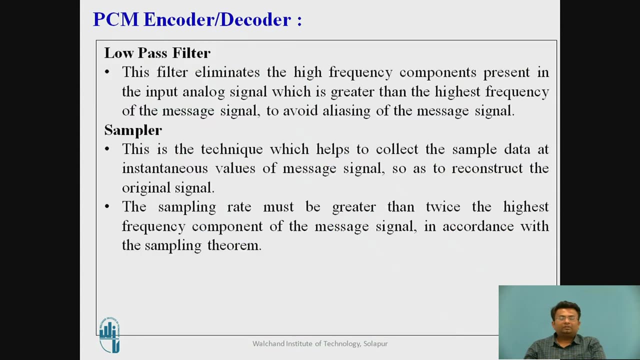 CD quality audio format. In this the 16-bit linear pulse-coded modulation technique is used for the quantization and the sampling rate is 44100 Hz. This is a block diagram of the PCM encoder and decoder. So these are the steps. The low pass filter: This filter eliminates the higher frequency. 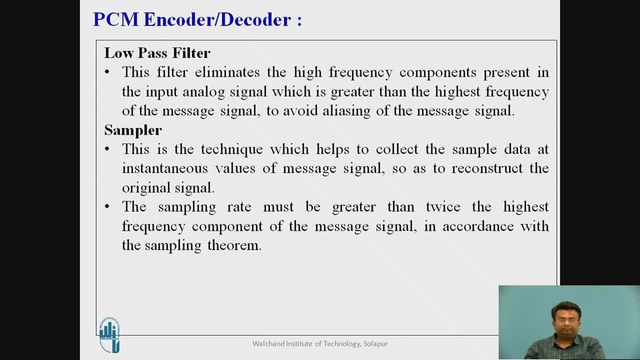 component which is present at the input analog signal, The sampler. This is the technique which helps to collect the sampled data At the instantaneous value of the message signal. So, in order to reconstruct the original signal, the sampling rate must be greater than twice the highest frequency component of the message signal, in accordance with the sampling. 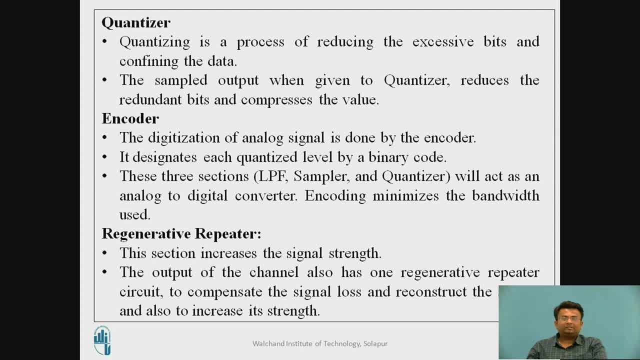 theorem Quantizer. Quantizing process is used in order to reduce the excessive bits and confining the data. The sampler output, when given to the quantizer, reduces the redundant bits and compresses the value Encoder: The digitization of analog signal is done by the encoder. 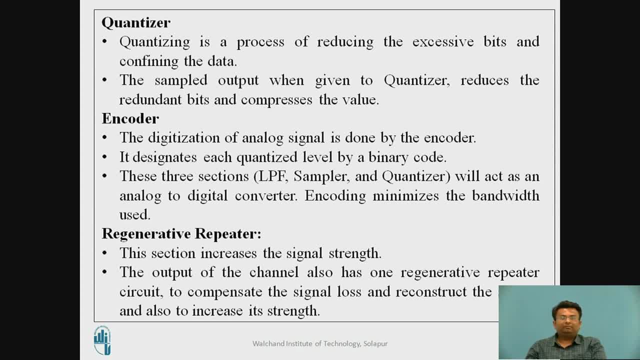 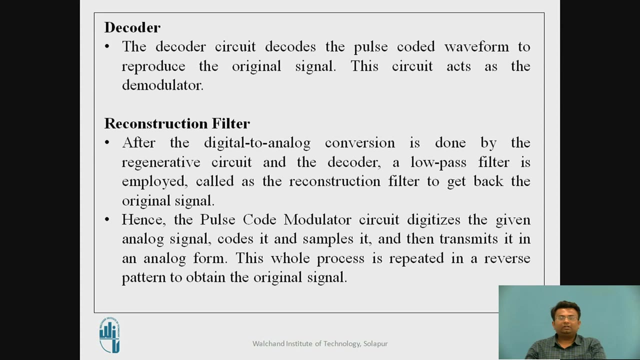 It designates each quantizer value by the binary code. Regenerative repeater: This section increases the signal strength. The output of the channel also has one regenerative repeater circuit To compensate the signal loss and reconstruct the signal And also to increase its strength. Decoder: The decoder circuit decodes the pulse-coded. 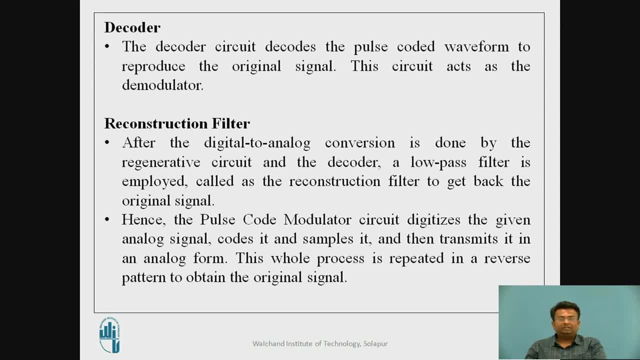 coded waveform to reproduce the original signal. This circuit acts as a demodulator. After the digital-to-analog conversion, which is done by the regenerative circuit and decoder, the low-pass filter is employed, which is called as a reconstruction filter. 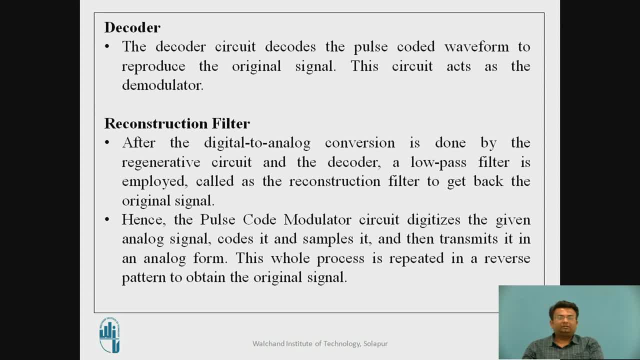 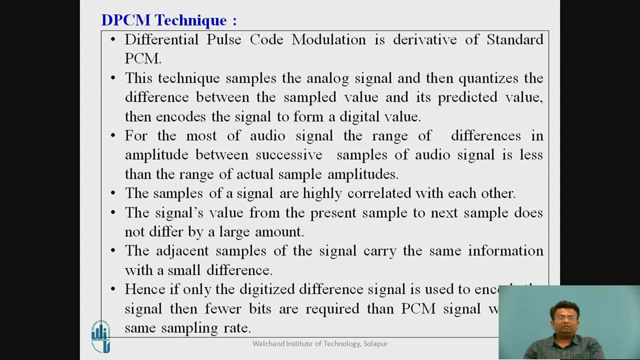 Pulse code modulator circuit digitizes the given analog signal, codes it and samples it and then transmits it in analog form. This whole process is repeated in a reverse pattern to obtain the original signal. DPCM technique: A differential pulse code modulation technique is a derivative standard of the pulse-coded modulation technique. 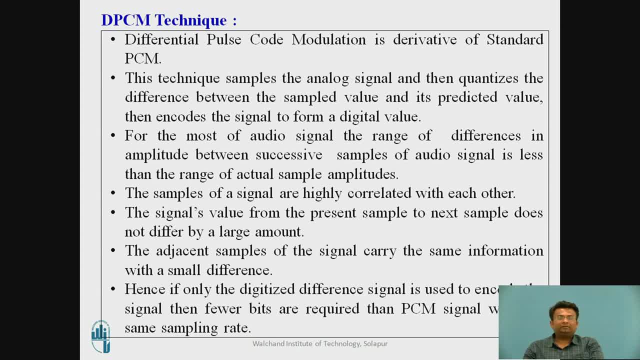 This technique samples the analog signal, then quantizes the difference between the sampled value and its predicted value, then encodes the signal to form the digital value For most of the audio signal. the range of differences in amplitude between successive samples of the audio signal is less than the range of actual 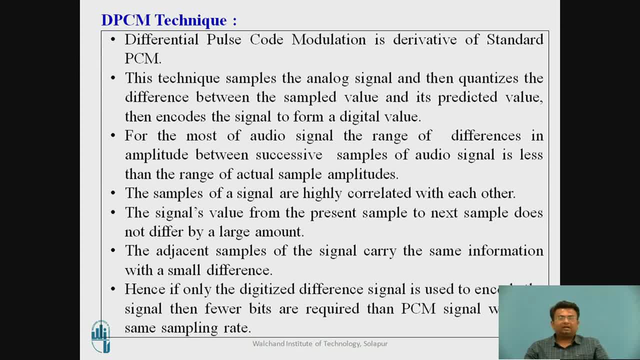 sample amplitude. The samples of the signal are highly correlated with each other. The signal's value from the present sample to the next sample does not differ by any large amount. The adjacent samples of the signal carry the same information with the small differences. Hence, if the difference between the values is digitized and encoded, then fewer bits. 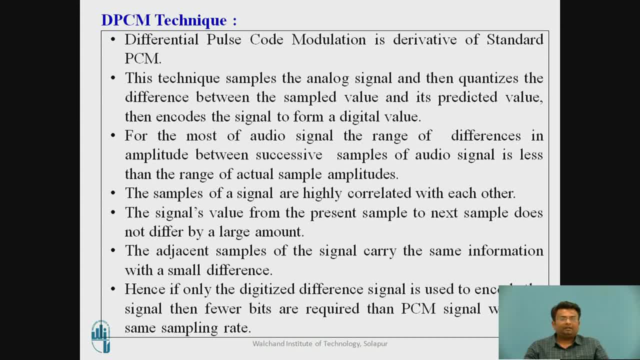 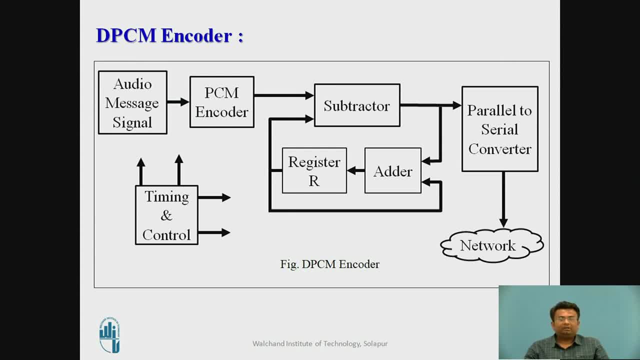 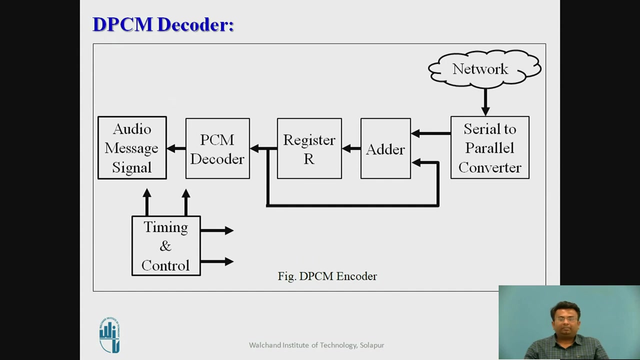 will be arranged to serial to panel parallel converter. so this will convert that serial data into the parallel and then it is added with the predicted value of the register and then this added value is decoded by the PCM. 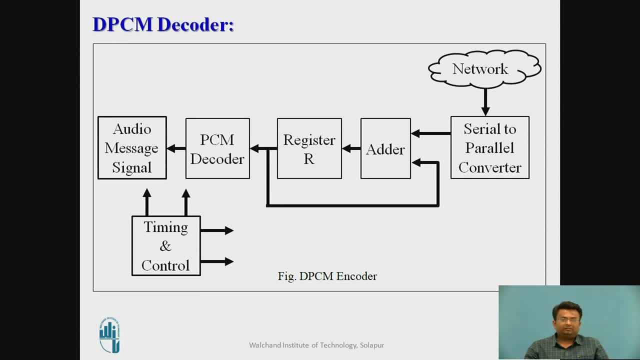 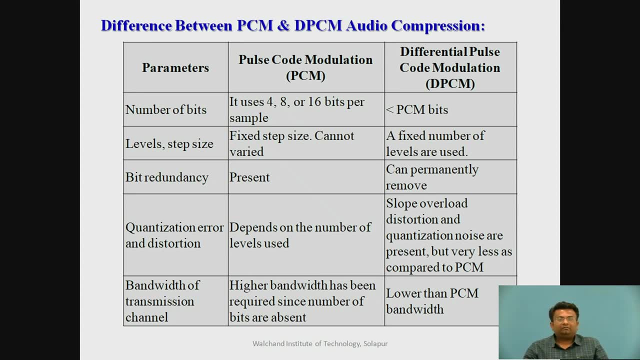 decoder and we will get the audio message signal. so what is the difference between the PCM and DPCM audio compression? the number of bits which is required for the PCM uses 4, 8 or 16 bit per second sample where, in case of the differential pulse code modulation less than that of the PCM. 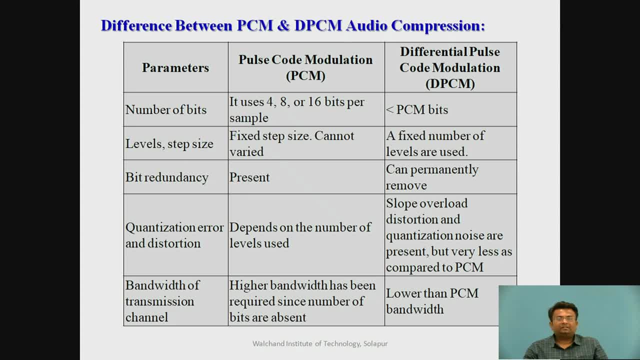 bits are required. step size: the fixed step size is used in this PCM modulation technique. here the fixed number of the levels are used. a redundant bits are present. it can be removed permanently in case of the DPCM quantization error and the distortion. it depends on a number of levels which are used and 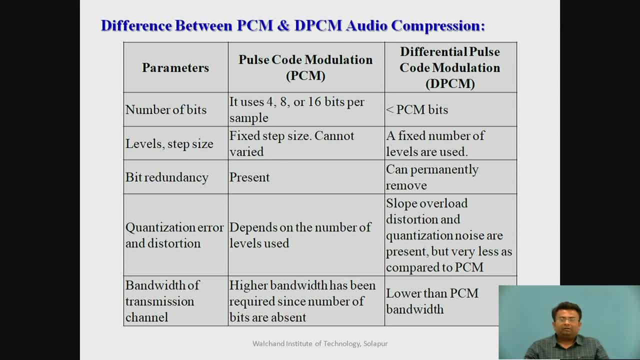 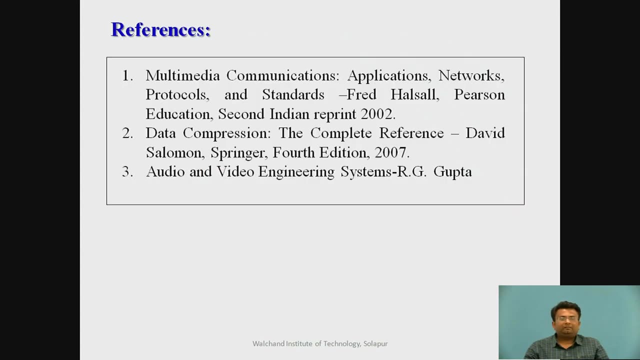 here. in case of the DPCM slope, overloaded, distortion and quantization noises are present, but very less as compared to the PCM. the bandwidth: the higher bandwidth is needed for the PCM and for the DPCM a lower bandwidth is needed. so these are the references which are used for the session. thank you. 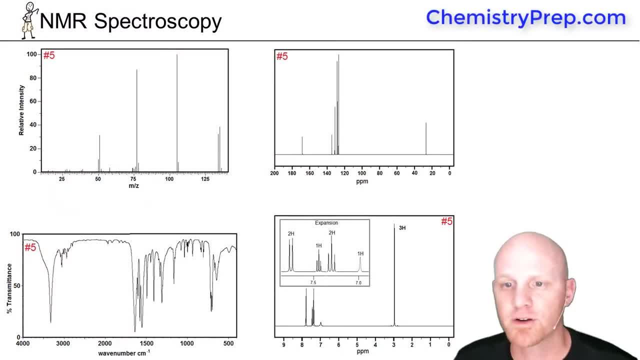 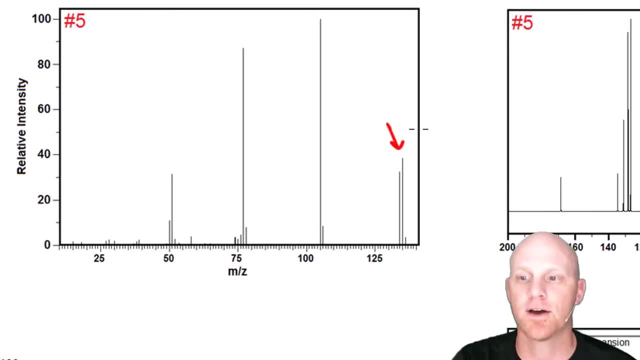 Okay, we're going to take the same approach here and look at the mass spectrum, then the IR, then the carbon-13 NMR, then the proton NMR And the mass spec. first thing I want to find is that molecular ion peak. So in this case we see that our molecular weight here is 135. And as I see, 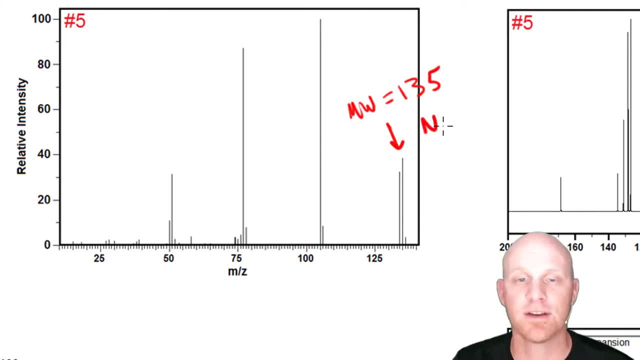 that's an odd number. bells should go off in your head And right off the bat you should realize you have nitrogen in your compound. At the very least you have an odd number of nitrogens, most likely one, but I can't rule out three, five, seven, nine or any other odd number. 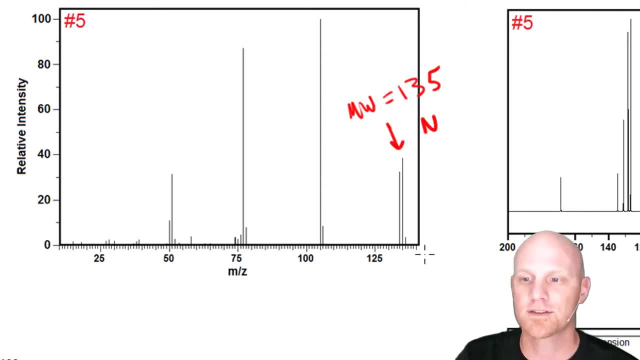 technically. But we do have nitrogen, with an odd number there, And in this case I'm looking for a peak at 137, and there's no significant peak at 137.. So I was looking for an M plus two and it's.